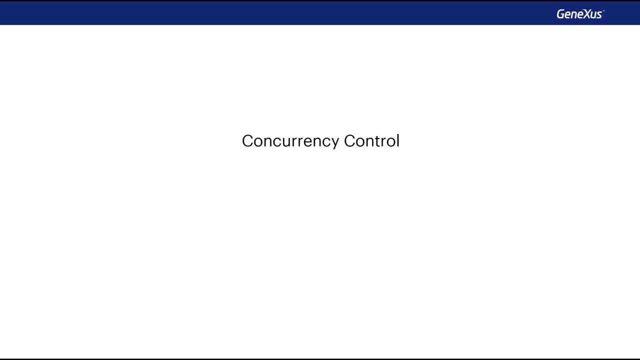 Let's start by looking at concurrency control in transactions and business components. Let's talk, then, about optimistic concurrency control. This mechanism assumes that multiple database transactions can be completed without affecting each other and that, therefore, these transactions can be performed without blocking the data resources involved. 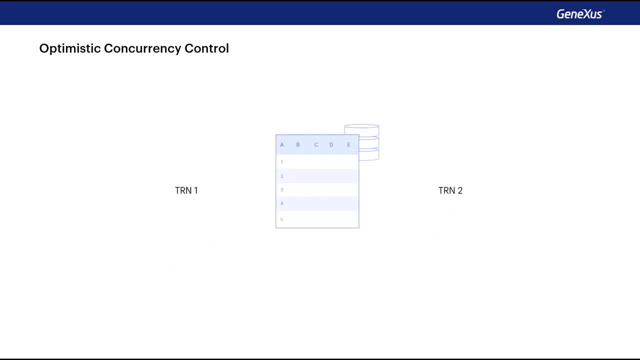 Before performing an update, each database transaction checks that no other database transaction has modified its data. This is related to the globalized nature of the web, where several users can access the same page at the same time. This makes blocking unfeasible for web user interfaces. 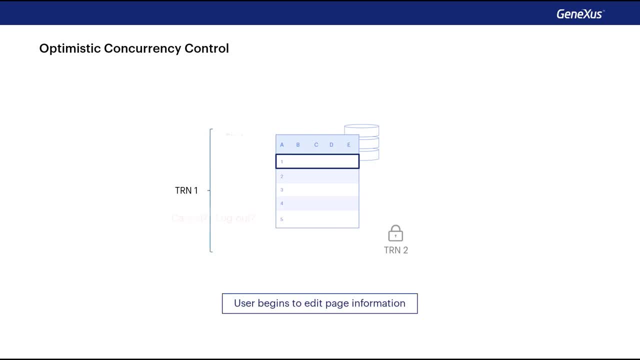 It's common for a user to start editing a record and then leave without following the cancel or logout link. If locking is used, other users trying to edit the same record must wait until the first logout. The first user's lock time expires. 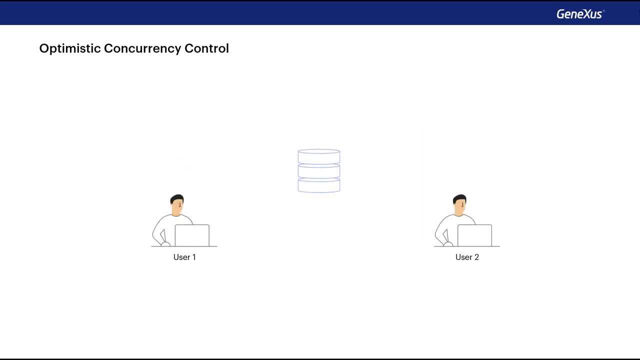 Instead of locking each record every time it's used, the system simply looks for signs that two users actually tried to update the same record at the same time. If such evidence is found, then a user's updates are discarded and the user is informed of this. 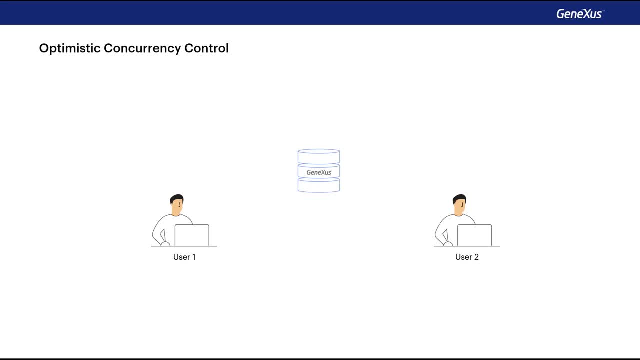 In GeneXus, when two or more users want to update the same record, the first one will be able to update it and the others will get an error because they were about to save new data based on outdated information that was updated by another user. 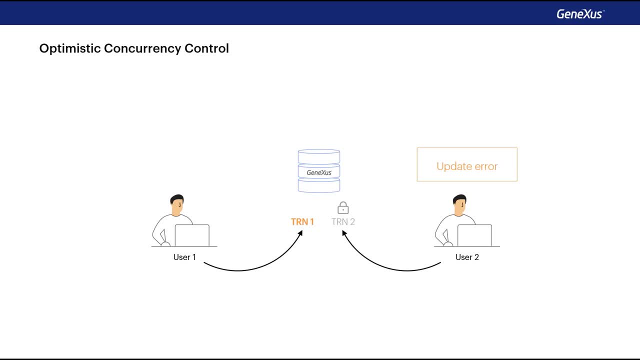 Then in these cases, the confirmation operation is reversed. The optimistic concurrency control is based on the old function. When a record is confirmed, the old values of each attribute are compared to the current values in the database, And if a value doesn't match, an error similar to the following is displayed: 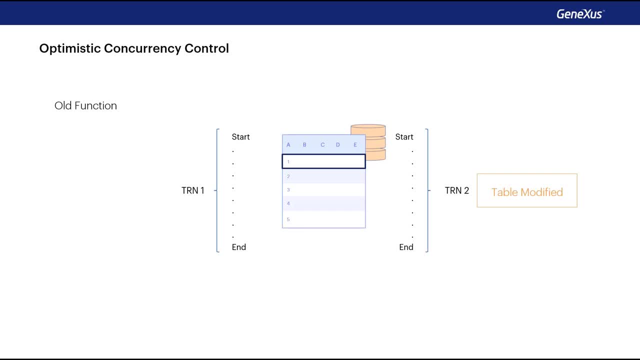 The table has been modified, which means that another user has modified the record since the values were obtained. It should be mentioned that only the attributes present in the transaction structure are taken into account. It should be mentioned that only the attributes present in the transaction structure are taken into account. 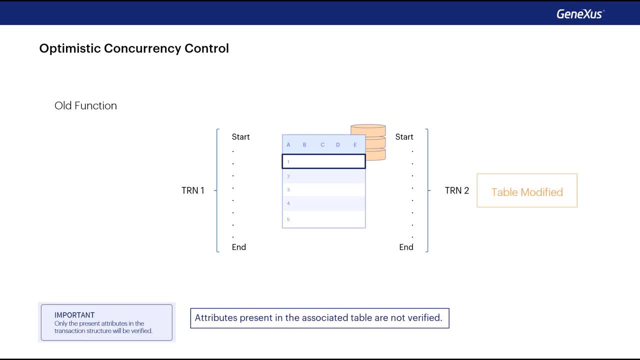 In other words, if there are parallel transactions with more attributes, they are not verified. This mechanism does not apply to attributes of types such as image, video, audio, longvarchar, nor to those attributes inferred from the extended table that are updated by means of rules declared in the transaction. 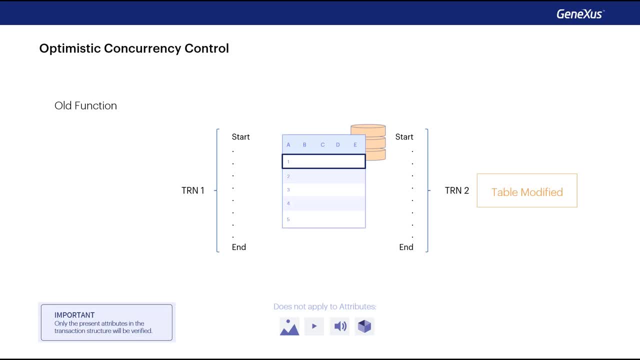 It only applies to attributes that are not part of the key. It only applies to attributes that are not part of the key Because the record is instantiated with them. Now let's see what Concurrency Control looks like in other GeneXus objects. 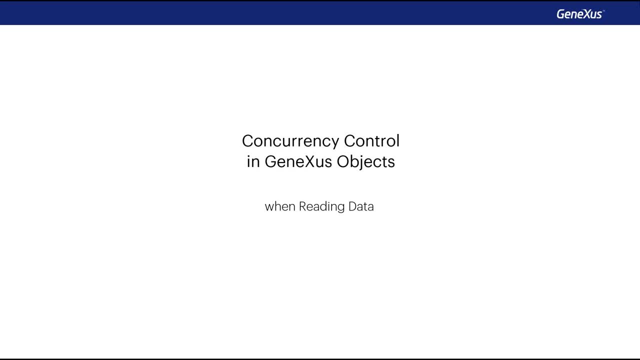 For example, how GeneXus handles locks when only reading data and when reading and writing data to control concurrency. What happens when data is only read? What happens when data is only read If it's read-only? when using foreach commands. webpanel-type object. 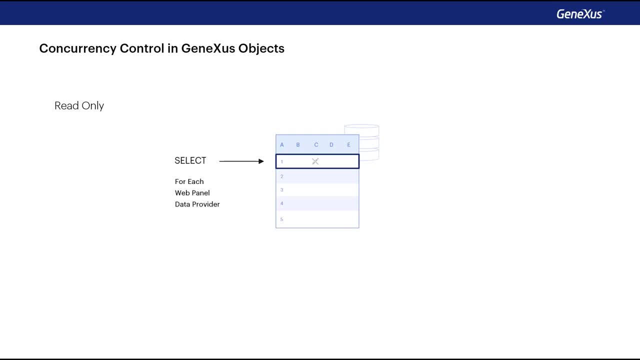 If it's read-only. when using foreach commands- webpanel-type object. What is the processing function for each command? webpanel-type object? objects, data providers and so on. the generated selects are not locked. They're always affected by exclusive locks. For example, in reorganizations, tables are 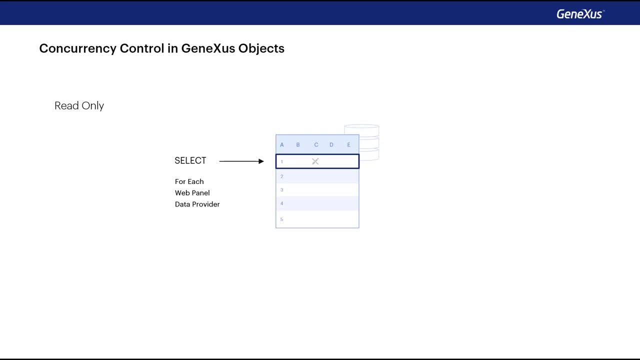 opened in an exclusive way. In this case, no other process will be able to open the table, no matter if it's read-only. On the other hand, if the information to be read is locked by another write program, the values to be displayed will depend. 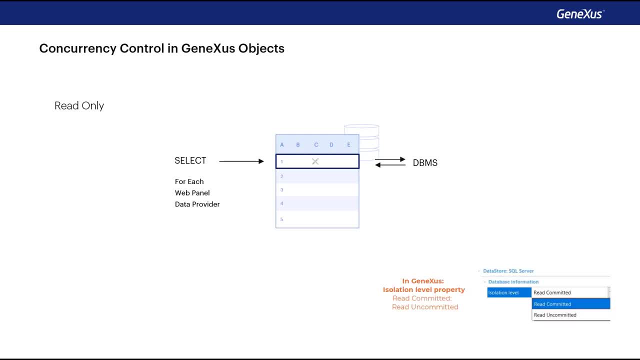 on the DBMS. It's then up to the DBMS to decide whether to display the old or the new value, And what happens when data is read and written. A foreach command that includes an update to the database performs a select with a lock when 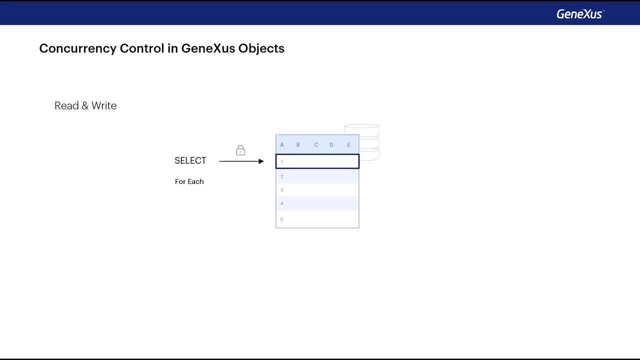 entering the foreach, and then the update is performed As any lock. it releases data to the database and then the update is performed As any lock. it releases data to the database, and then the update is performed As any lock it releases.